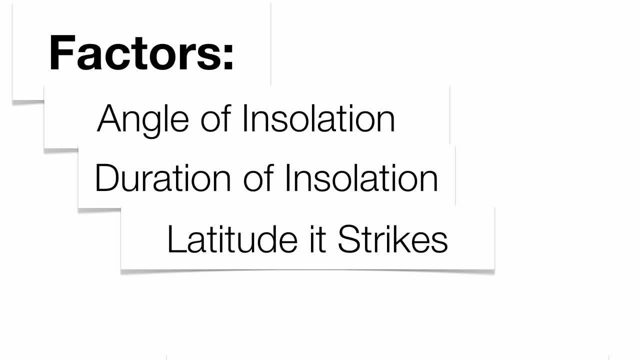 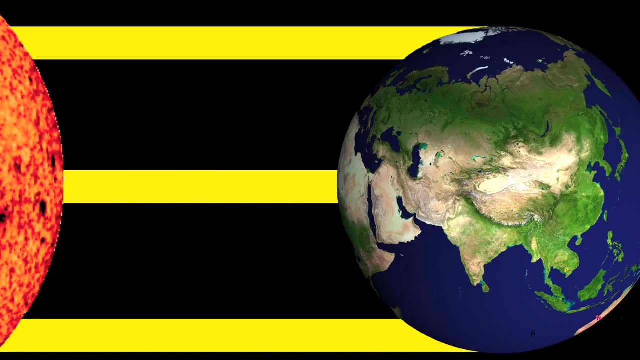 strikes is going to be important. North Pole and South Pole are much colder than the equator And the strength of insulation- The higher the angle, the greater the intensity. The lower the angle, the weaker the intensity. So you'll see that the North Pole and the South Pole have much lower angles and they have much 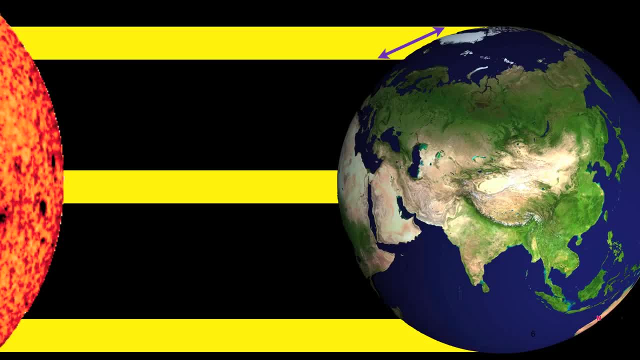 weaker intensity from the sun. That's why it's quite cold. You'll see how wide that light beam is when it strikes the surface, Compared to the equator, where it's much more direct. that angle right there is about 90 degrees to the surface. It's much more compact. it's much. 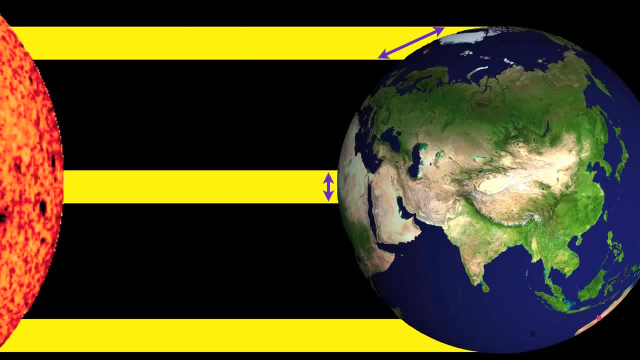 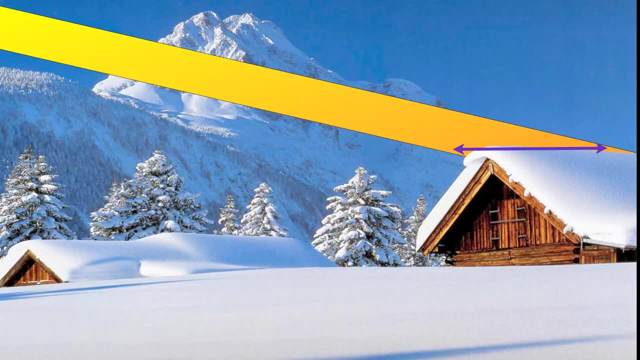 more direct. that's why it's much warmer at the equator compared to the poles. So the sun's energy coming in, That's a much, much lower angle of insulation. You see how wide that light beam is. add that leads to lower temperatures, lower angle and lower intensity energy from the. 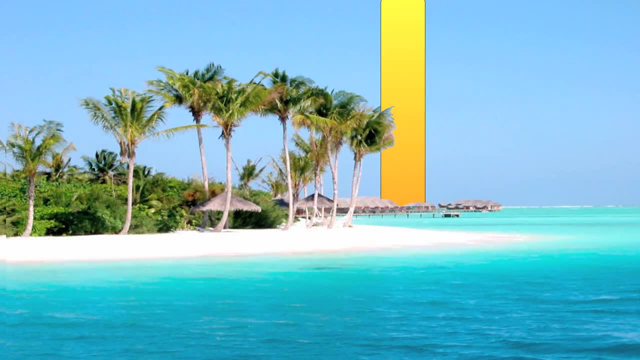 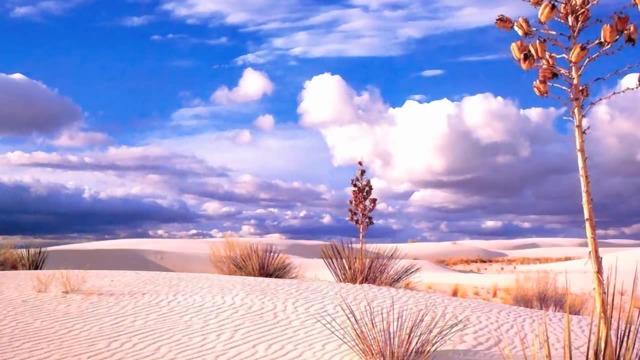 sun. Compare that with the equator, where it's much more direct, much more compact, higher angle, greater intensity, higher temperatures. Not only with latitudes does that change, but also through the course a day, You can see. in this case, my afternoon sun is pretty close to 90 degrees. 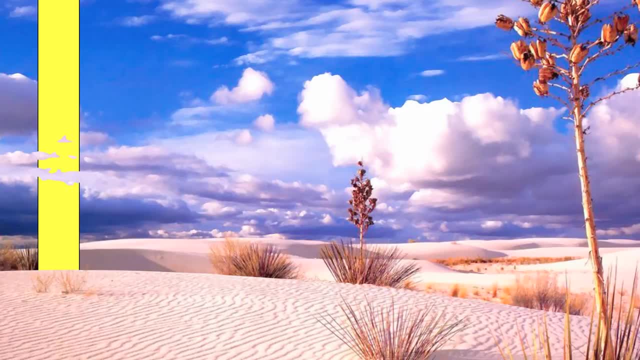 That's gonna be a very direct ray. It's gonna put light into the equator and that's gonna save my sun, going to probably give me some pretty hot temperatures through the course of the day. Now, either the sun rising or the sun setting, you'll see that the light beams coming in from 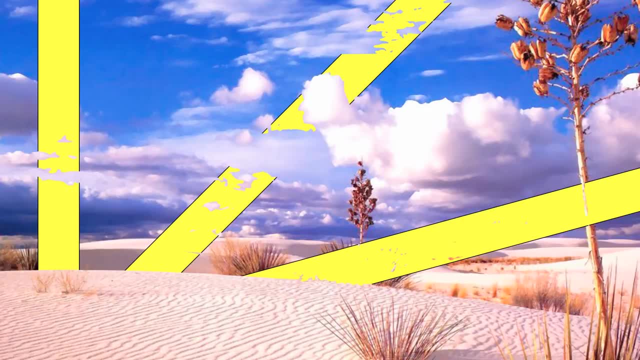 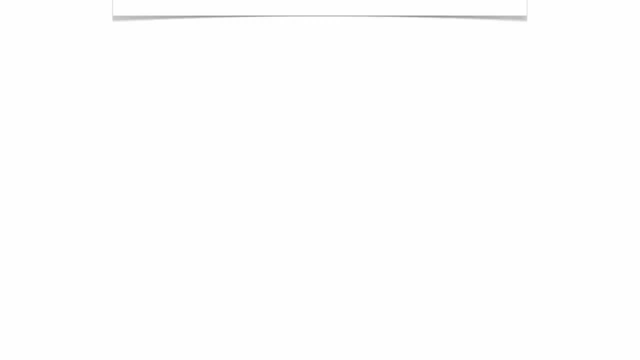 the sun are significantly lower. Lower the angle, lower the intensity, lower the temperature. So your morning and evening are a little bit cooler than your afternoon, all because of the angle and the intensity of the sun. Now you have a couple important dates here. You have the first day of 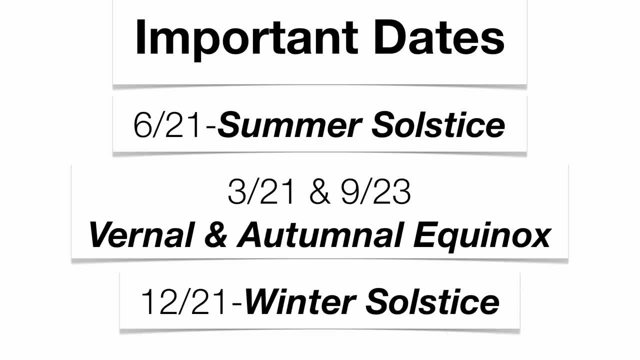 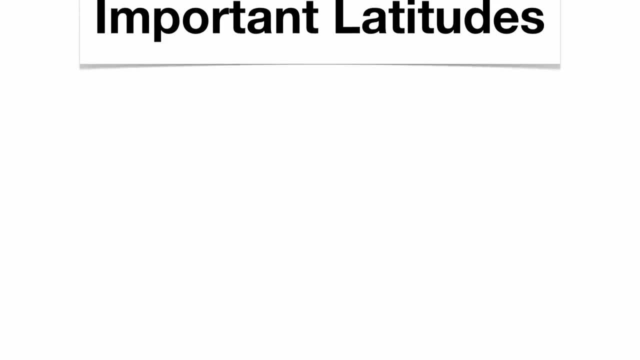 summer, the first day of spring, the first day of fall and the first day of winter. They all have specific names to them, so make sure you know the names of those important dates. Now, those dates have certain latitudes that you need to associate with them. The reason is because you need to know. 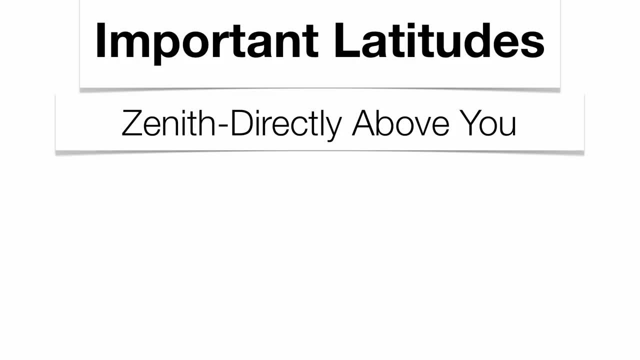 where the sun is going to be at the zenith on those four basic dates. The zenith is going to be the point directly above you, giving you sun's energy at about a 90 degree angle. So on June 21st, the Tropic of Cancer is going to have the sun at the zenith On March 21st and September 23rd. 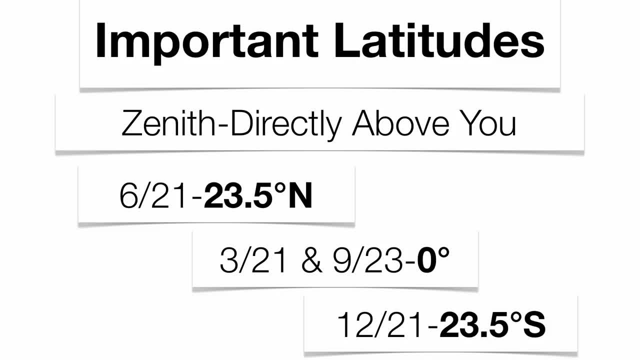 the equator is going to have the sun at the zenith And then, December 21st, the Tropic of Capricorn, the sun is going to be at the zenith there. So you have four dates, three latitudes, because your two equinoxes are going to double up with the equator. 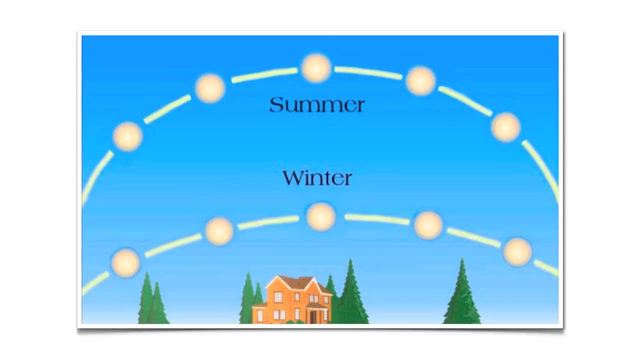 Four dates, three latitudes you need to know. Now you see that the sun's path varies significantly between summer and winter. Summer it's got a much higher angle of insulation, much more intense energy, It's out for a longer period of time, which gives you hotter temperatures. The winter 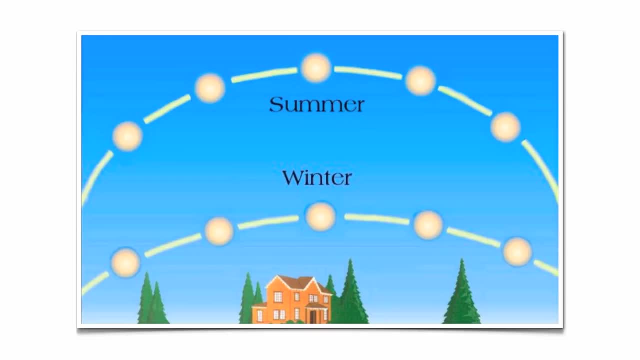 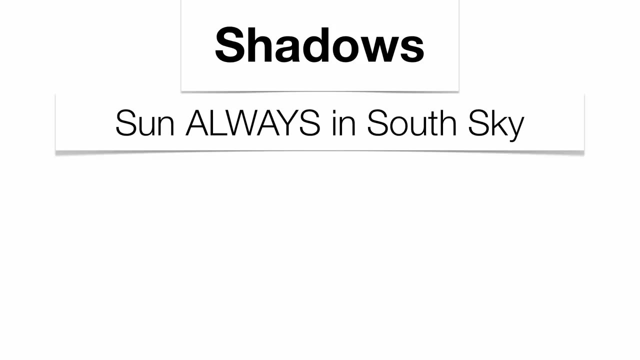 angle gives you much lower intensity light, which gives you the colder temperatures. Now shadows are going to be important. They always tend to be asked on your regions exams. You have to realize that the noon sun's always in the southern sky here in New York State. 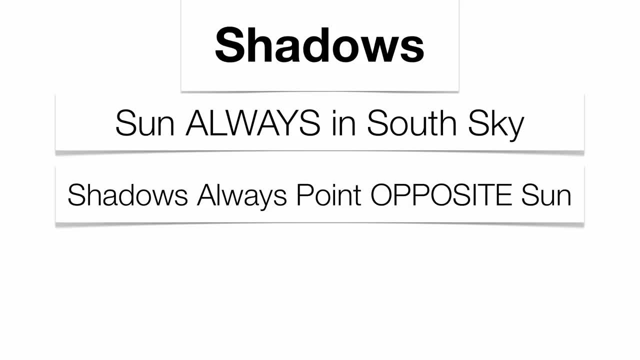 which means that your shadow is always going to point in the opposite direction. So, whether or not the sun is in the east, if it's in the southern sky or if it's setting in the west, realize that your shadow always points in the opposite direction of the sun. Your shadow length. 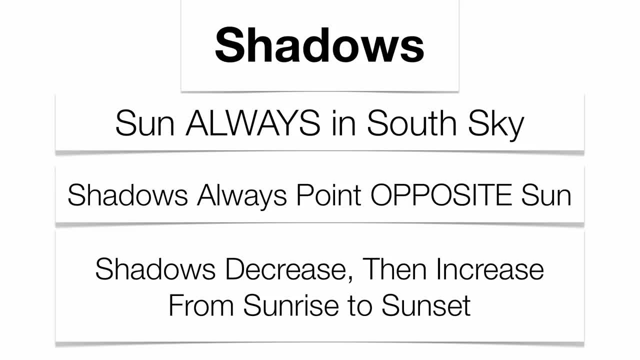 is going to vary as well. From the north to the south it's going to vary as well. So you have to realize that from sunrise to sunset it's going to get smaller as it gets up to noontime and it's. 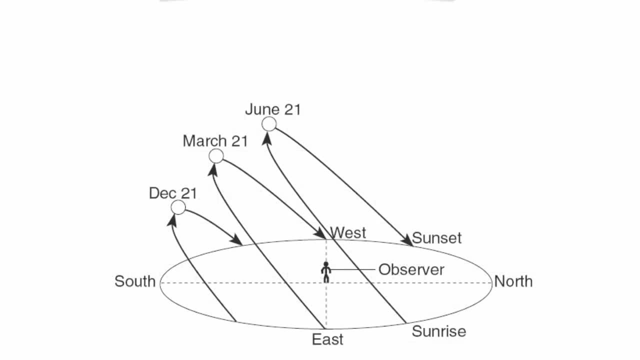 going to get larger as it gets down to sunset. Now here's a classic diagram from the regions that shows you your four basic dates, Remember March 21st and September 23rd. they double up of the sun's path And what we're going to do is we're going to take this diagram and we're going 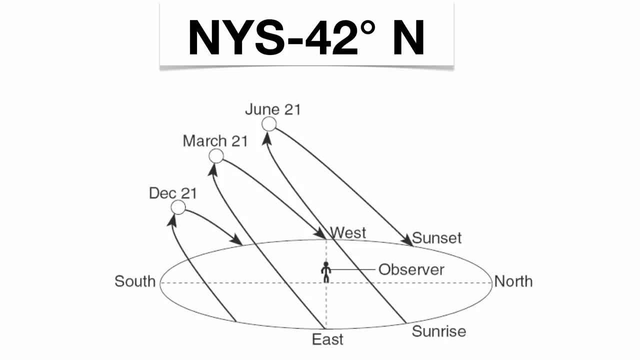 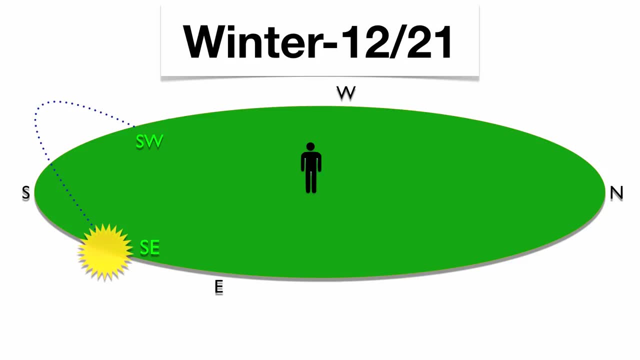 to break it down season by season. You definitely need to have an idea about what this diagram actually means. So the first date's going to be your winter solstice. You'll notice that the sun is rising in the southeast. You'll notice that the sun is rising in the west. You'll notice that the 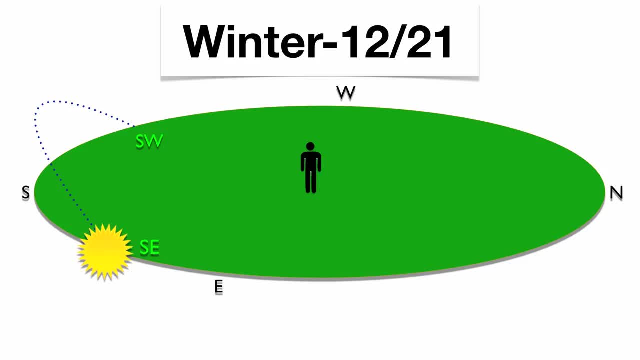 sun is setting in the southwest. It's only out for about nine hours out of the day. Now, when that sun rises up, your shadow's going to be pointing in the opposite direction of the sun. That sun's going to get to a maximum altitude of about 24 and a half degrees above the horizon. You'll notice. 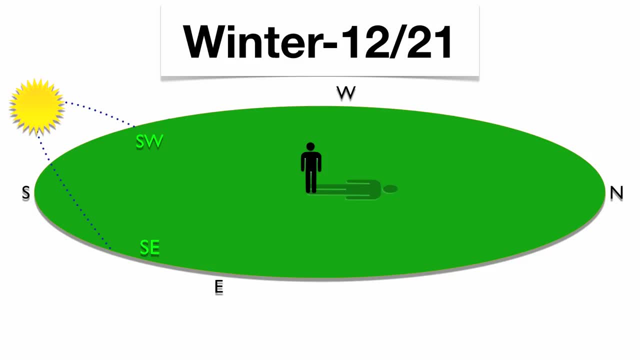 that the shadow length just got smaller And you'll notice that my noontime sun the shadow's pointing in a northerly direction. As that sun sets in the southwest, the shadow always points in the opposite direction and gradually gets longer as well. 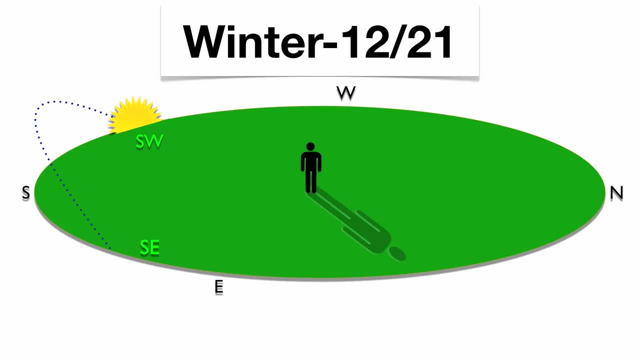 Because of the lower angle of insulation. So, regardless of the season, your wintertime sun is going to be out for the shortest period of time and has the lowest angle of insulation because it has the lowest altitude, only about 24 and a half degrees above the horizon. So when you take a look here at the shadow and you also take notice that, 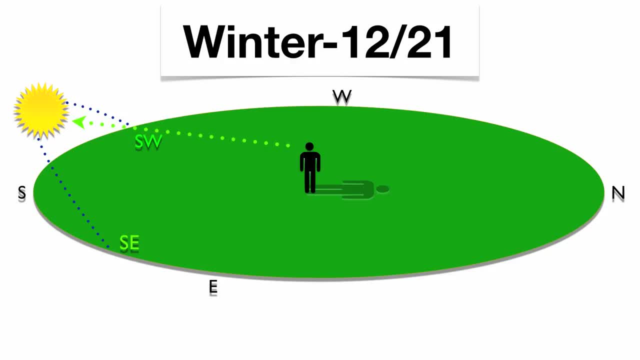 your observer here is looking at the sun in the southern sky. your shadow's going to be pointing north. Now just take note of the length of the shadow. It's going to be about noontime in winter and we're going to try to compare that, try to remember that- what the shadow looks like when we get to the summertime. 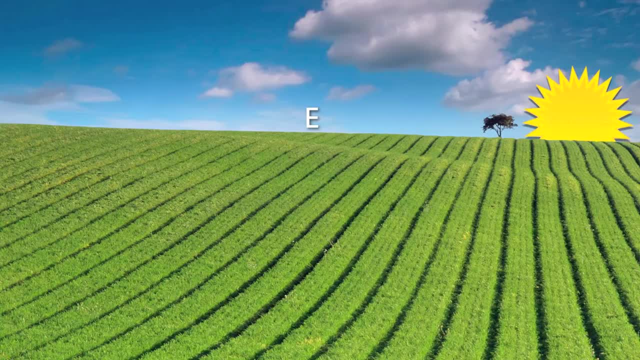 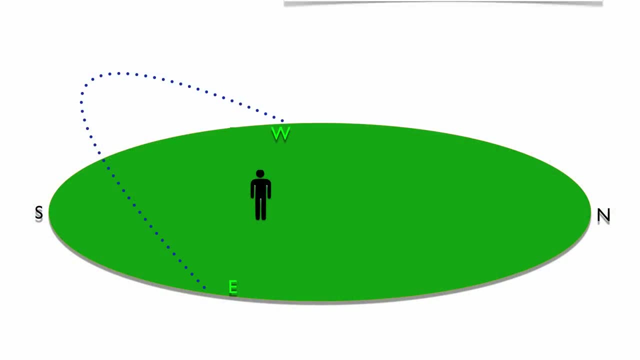 Now my sun is going to rise in the southeast part of the sky and that's going to be where my wintertime sun's going to rise. It's only going to be out for about nine hours out of the day. Then I get to fall and spring, which are my autumnal and vernal equinox. You'll see that my sun is going to be rising exactly east and setting exactly west. 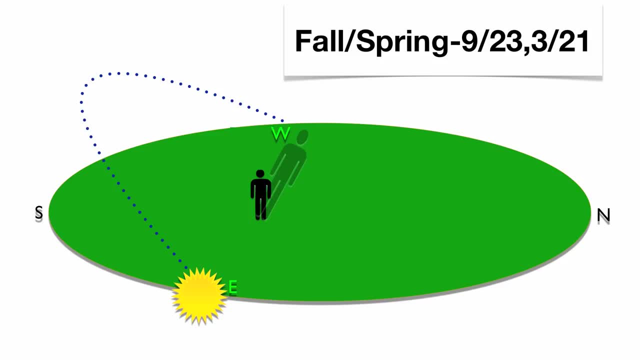 My altitude is at a 48 degree angle now. You'll notice that my shadow is going to get smaller as it gets noontime, so take note of the shadow length and the shadow direction, and then also when it sets. Now my sun is going to be out for 12 hours on this day, across the entire. 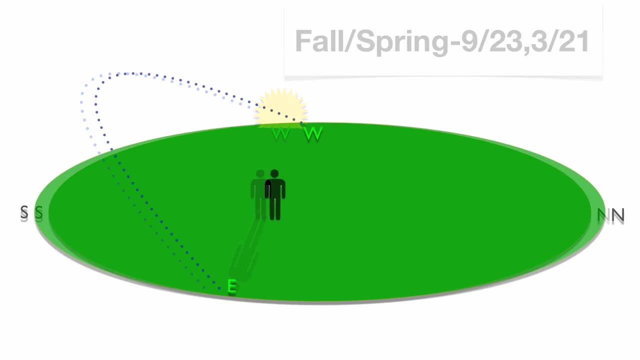 planet. Now that person, again for fall and spring, needs to look in a southerly direction. Notice that my noon shadows a little bit smaller than what it was in wintertime because my angle of insulation is a little bit greater. 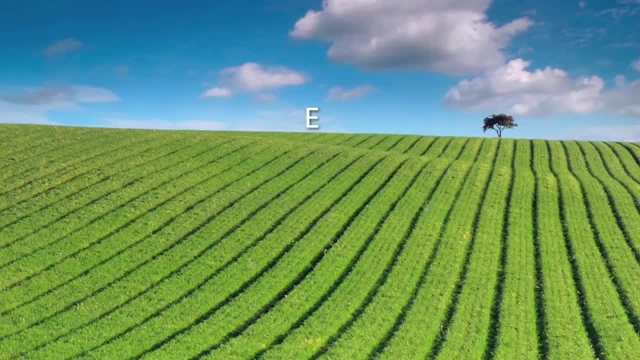 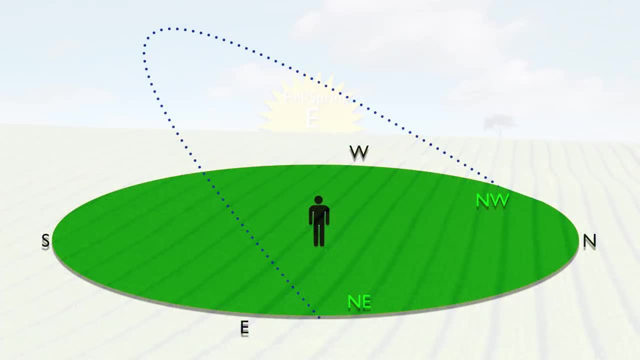 now Again, my Sun's gonna rise exactly east and set exactly west for fall and spring. Now summertime, it's gonna be my summer solstice. Now you'll notice that my noon Sun will not hit the zenith, will not be directly above the observer, but 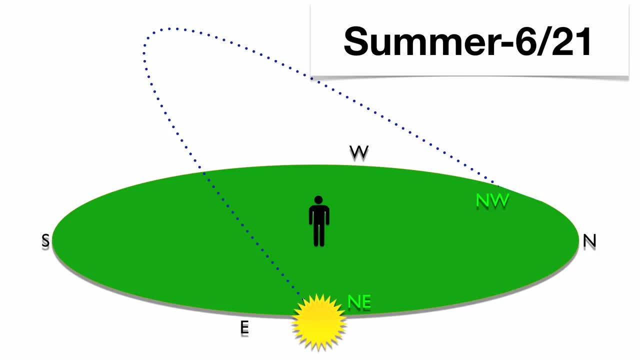 it's gonna rise in the northeast. it's gonna take a very long path, 15 hour path now, across the sky. My shadow is pointing opposite. Now watch what happens to my shadow length Significantly smaller. So, even though at noontime for every day of 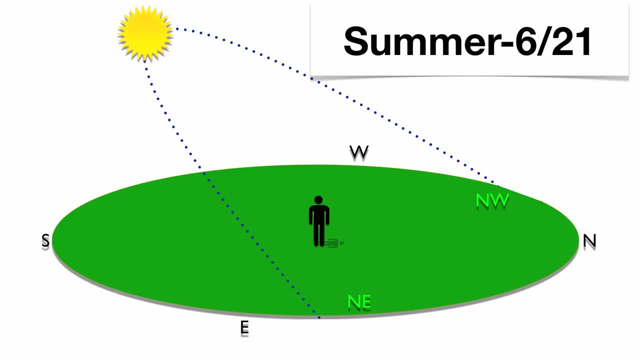 the year. your smallest shadow is gonna be at noontime. If you compared your four seasons, summertime would be the shortest. wintertime would be the longest, because your Sun's altitude now is 71 and a half degrees above the horizon- Much more. 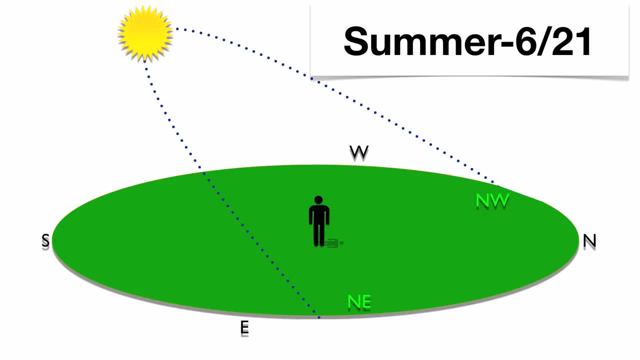 direct Sun, higher angle of insulation, greater intensity. here It's gonna set in the northwest. Notice the shadow gets longer at sunset and it points in the opposite direction of the Sun. Again, that noon Sun during summertime is gonna be in the southern. 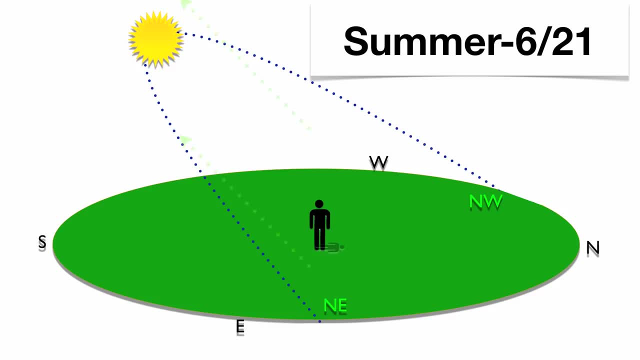 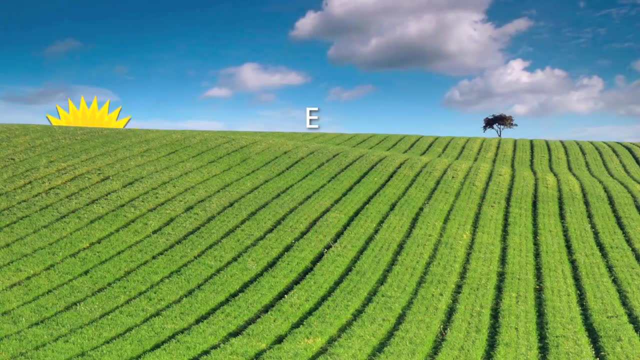 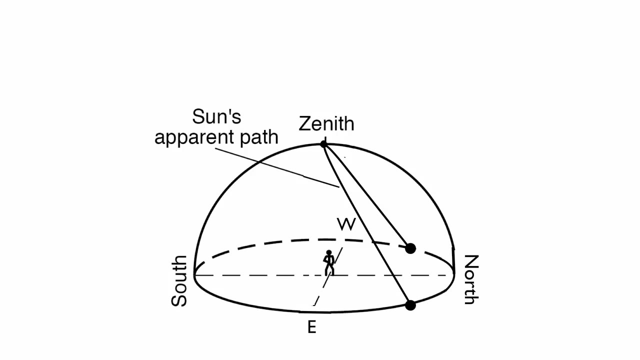 sky A really small shadow pointing north at noontime, and again you have a much, much higher angle of insulation here Again. now my Sun's gonna rise in the northeast part of the sky during the summertime here in New York State. Well, you also have. 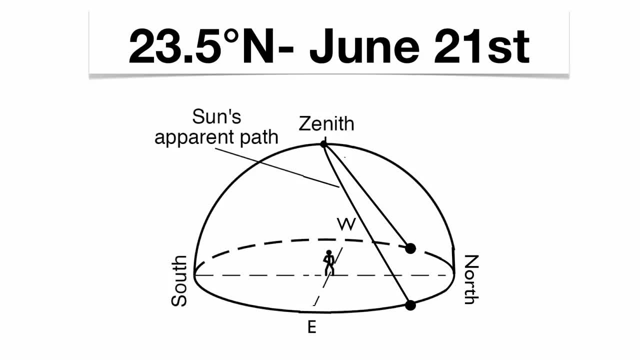 a couple other latitudes that you need to know. Well, this is significant because at 23 and a half degrees north- this is going to be June 21st- the Sun's gonna be at the zenith. You'll notice that that noontime Sun is gonna be directly above. 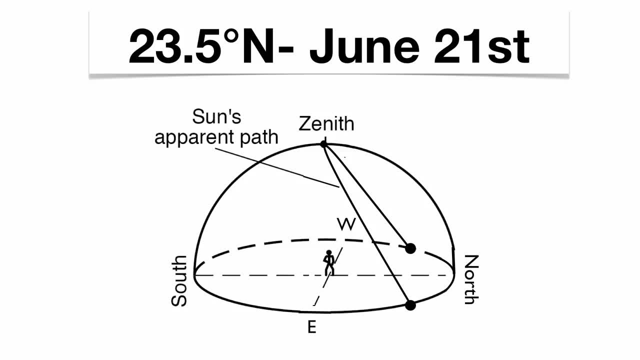 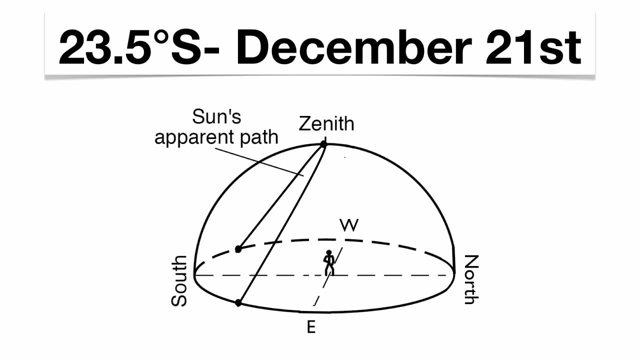 the observer. That's gonna be a picture that would be indicative of the Tropic of Cancer, and the Sun's gonna be at the zenith on that specific date. You'll notice that this is the Tropic of Capricorn. You'll notice now that the 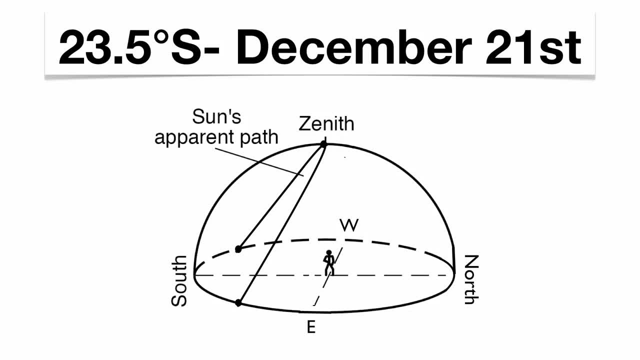 Sun is rising in the southeast and setting in the southwest. Everything's a little bit opposite in the southern hemisphere, but you'll notice this is going to be the latitude that gets the most direct Sun. on December 21st. The Sun is at the zenith. Reason for that? It's the southern hemisphere's summertime on. 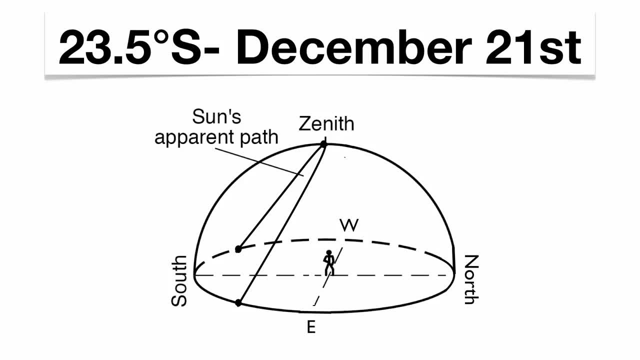 this date. Even though it's our first day of winter, it's going to be southern hemisphere's first day of summer. This is going to be what the equator looks like. This is going to be on March 21st and September 23rd. 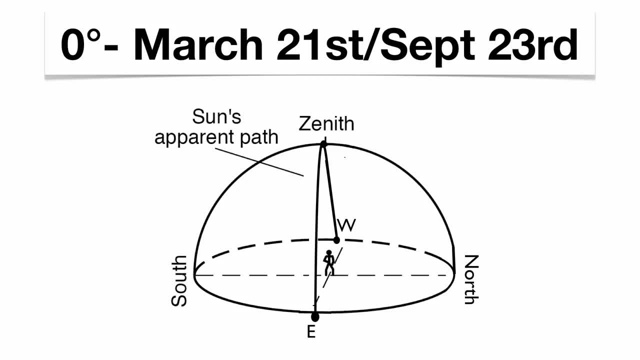 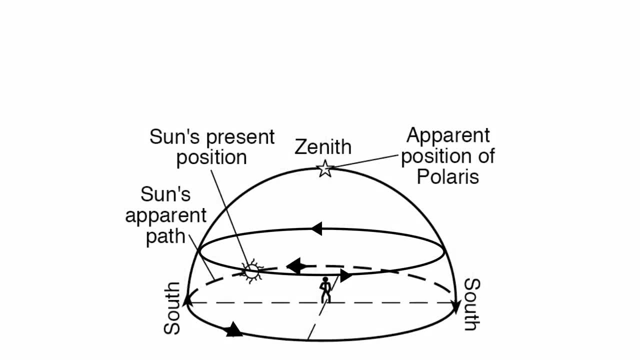 It's gonna rise exactly east and set exactly west, and the Sun's gonna be at the zenith on those two dates at the equator. Then, finally, this is gonna be the North Pole on March 21st and June 21st, You'll 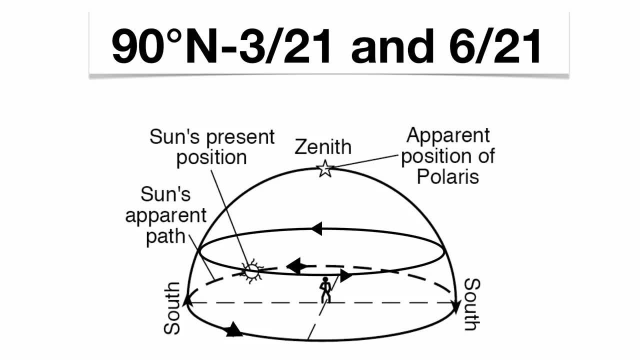 notice that there's two paths of the Sun that are being depicted here. Now you'll notice that there's no date here for December 21st, because the Sun is below the horizon. Okay, it doesn't come out. North Pole's in 24.